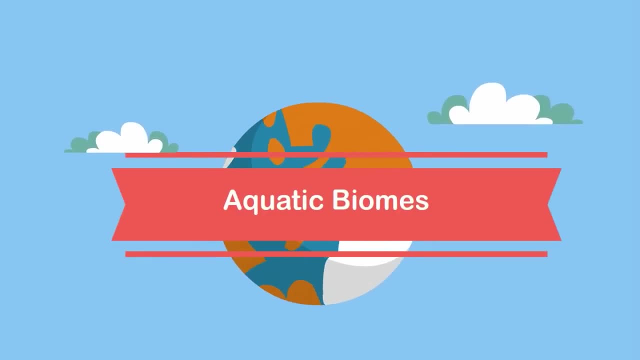 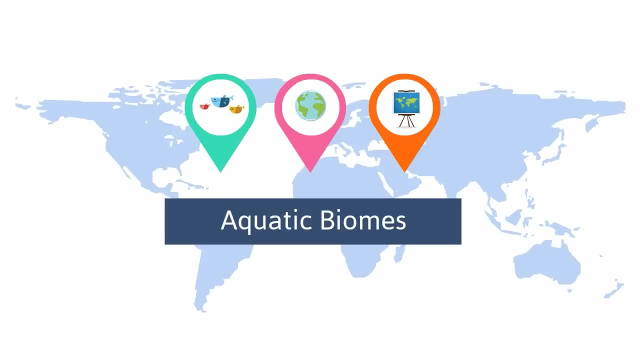 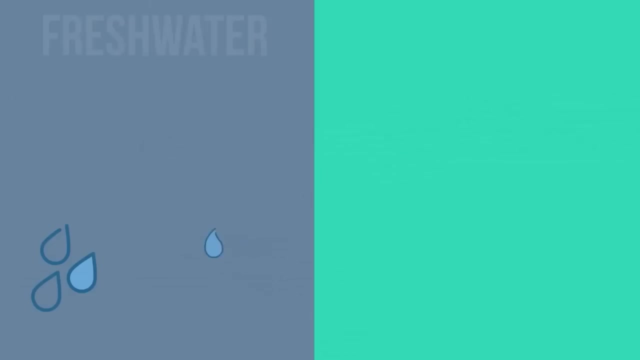 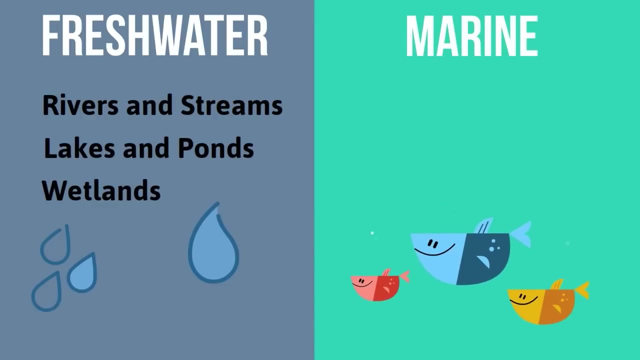 Welcome to MooMooMath and Science. In this video, I'd like to talk about aquatic biomes. The earth is made up of almost 70% water. This water can be divided up into two basic aquatic biomes. They are freshwater, which include rivers and streams, lakes and ponds and wetlands, along with the marine biome, which include the ocean and estuaries. 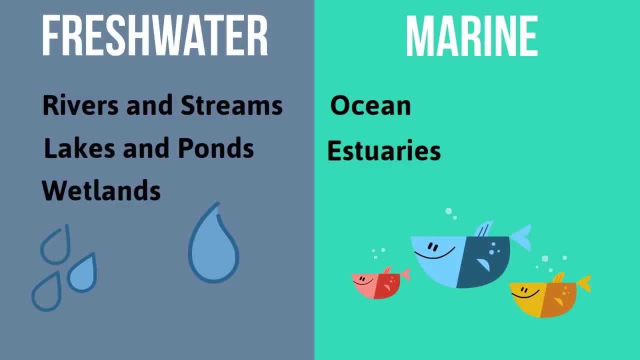 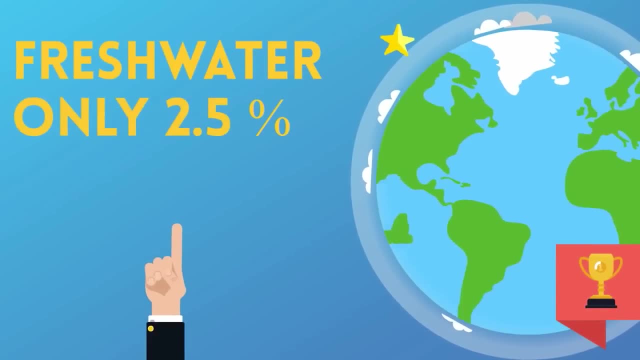 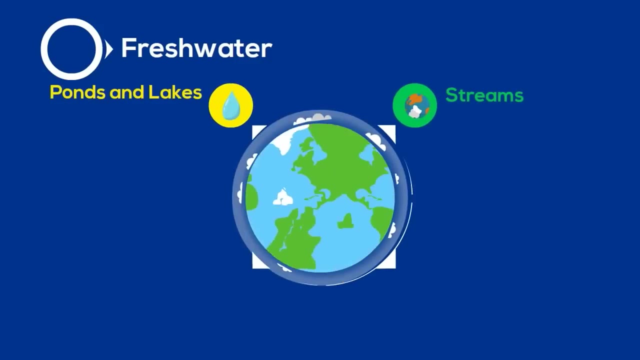 So let's get started with aquatic biomes. Let's talk about freshwater biomes. The earth has lots of water, but only 2.5% is freshwater. The major freshwater biomes include ponds, lakes, streams, rivers and wetlands. 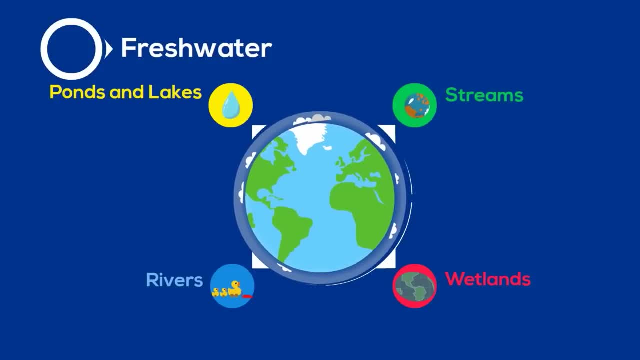 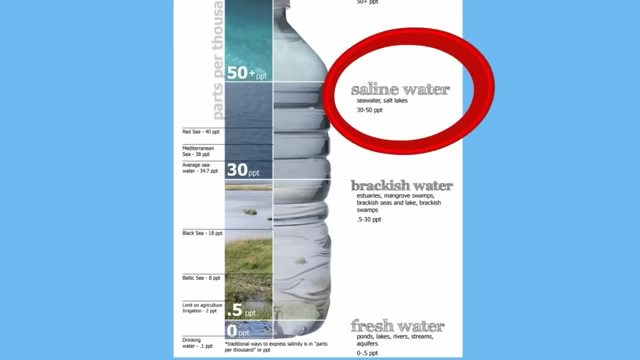 Plants and animals in these freshwater biomes are adapted to the low salt content in freshwater and are also adapted to the low salt content in freshwater. They are unable to survive in areas of high salt concentration. Saltwater is 30 to 50 parts per thousand salt to water, where freshwater is only 0.5 parts per thousand. 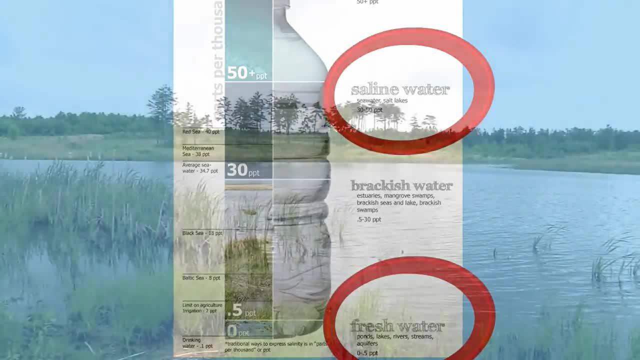 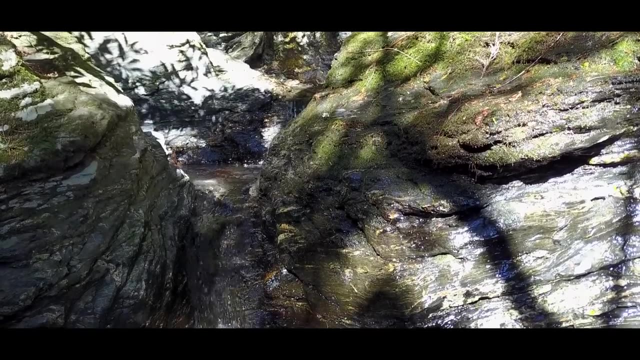 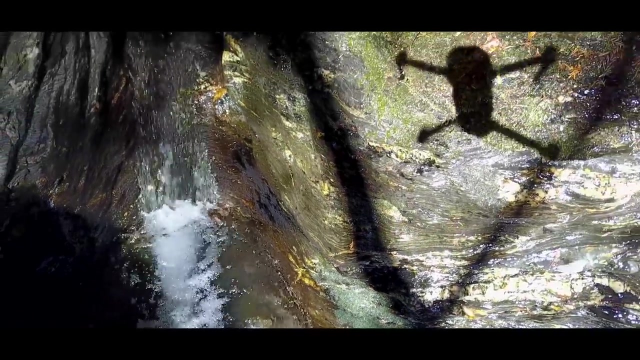 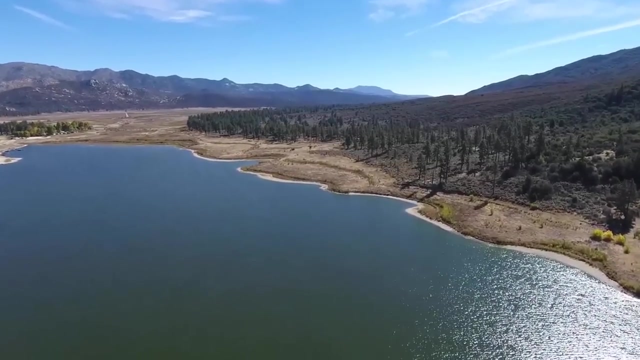 Let's take a look at some freshwater biomes. There are 12 different features of a freshwater biome. Number 2 is for67% sand pressure from 1500 to 1.1% of an acre per liter. Therefore, around the collective 2 types of water lifetime are available, the methodology of which includes characteristics such as water quality and nit��이하기. 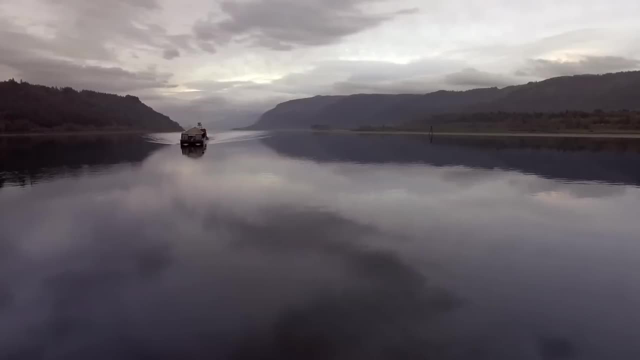 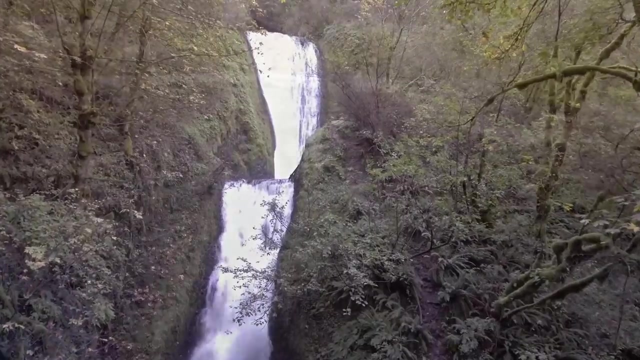 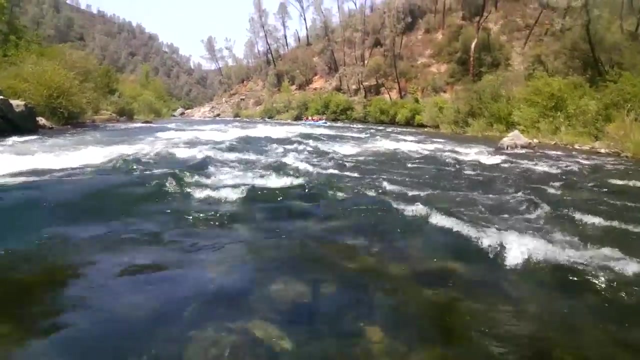 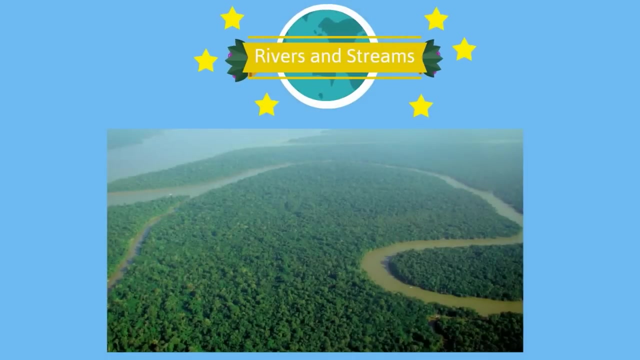 percentage of water hurdles. What are the different properties of freshwater biomes, Saltwater, Startup, tuna, Umeda, Bear, beight, Corey, Lifeide, Muna воды, Rivers and Streams. The water in rivers and streams flow in one direction, beginning at the source called a headwater and traveling to the mouth, where 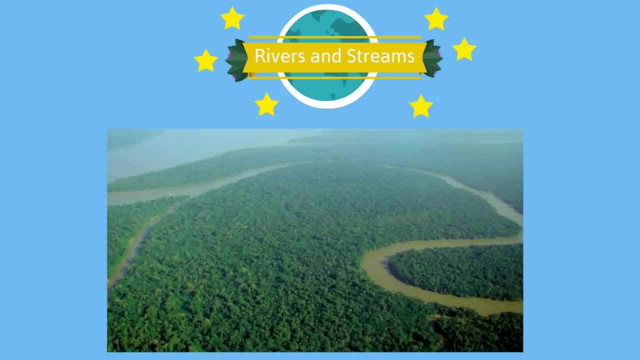 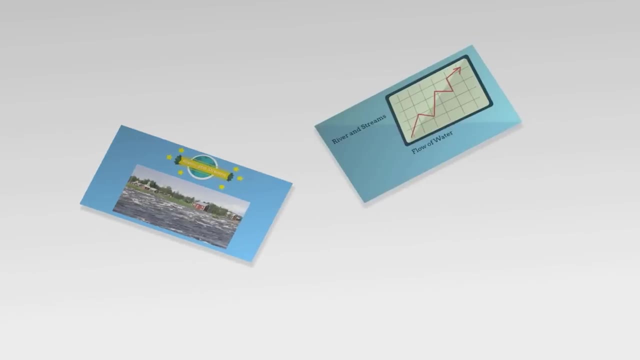 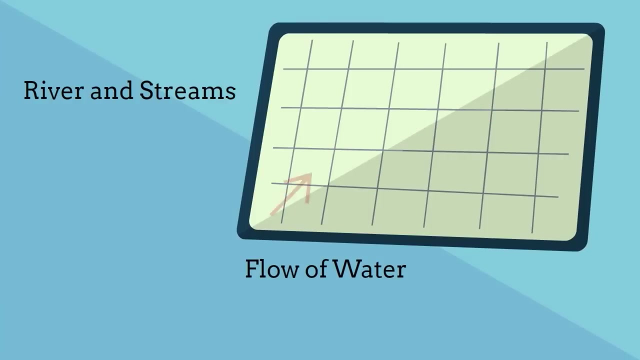 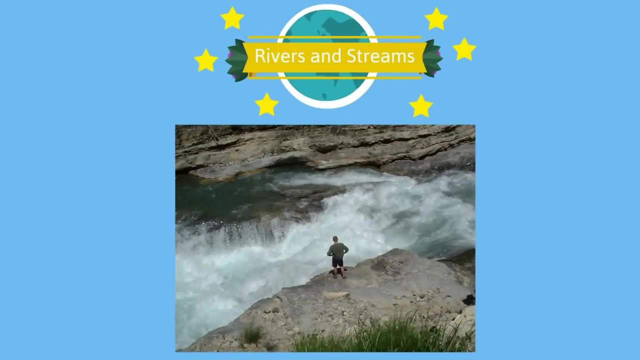 the flowing water empties into a larger body. The slope of the landscape determines the direction and speed of the water flow. When the slope is steep, water flows quickly. When it is not as steep, the water slows down. The currents and turbulence of fast-moving rivers and streams prevent much accumulation. 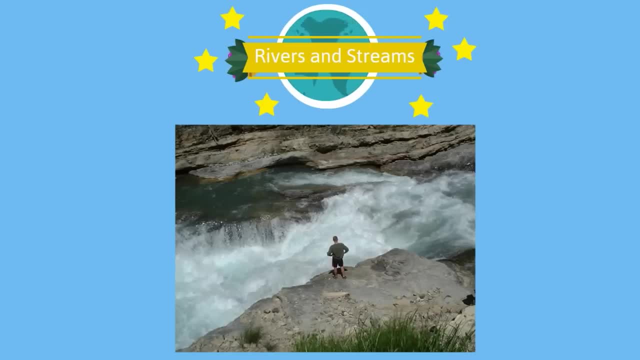 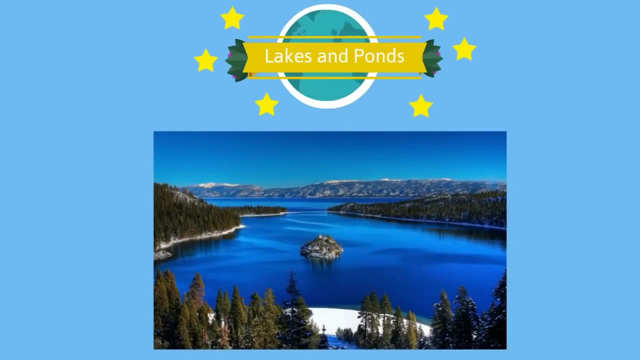 of organic materials in fast-moving rivers and streams. Lakes and ponds are inland bodies of standing water. It can be as small as a few square meters or as large as a thousand square meters. Some ponds might be filled with water for only a few weeks or months each year, whereas 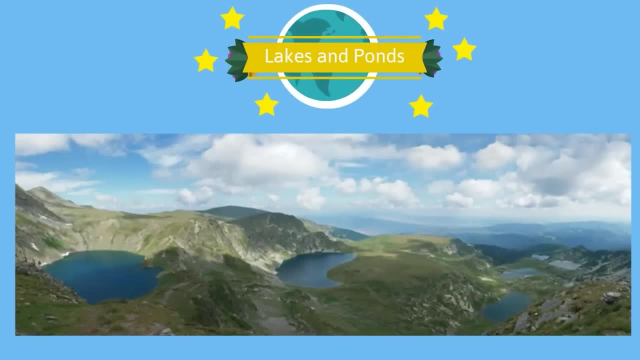 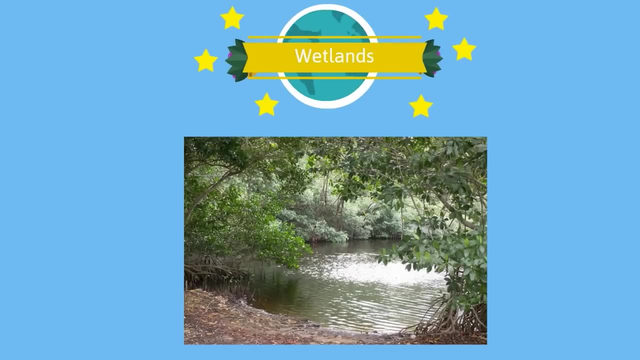 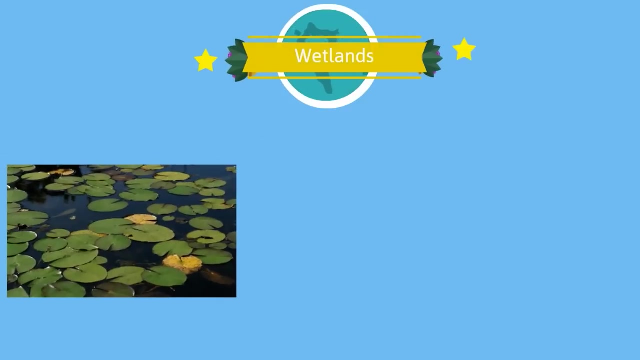 some lakes have existed for hundreds of years. Wetlands are areas such as marshes, swamps and bogs that are saturated with water and support aquatic plants called wetlands. Plant species that grow in the moist human conditions of wetlands include pond lilies, cattails and willows. Wetlands have a high level of species diversity. Many amphibians, including salamanders and reptiles and birds, live in the wetlands. Freshwater biomes. We have rivers and streams, Lakes and ponds And wetlands. The earth is roughly 70% water. 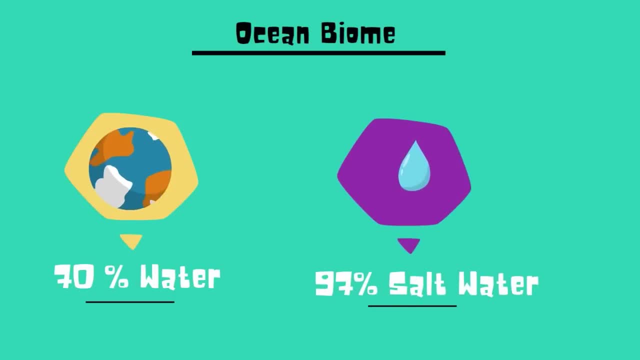 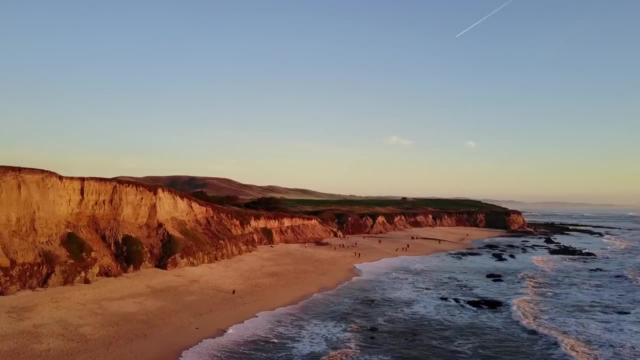 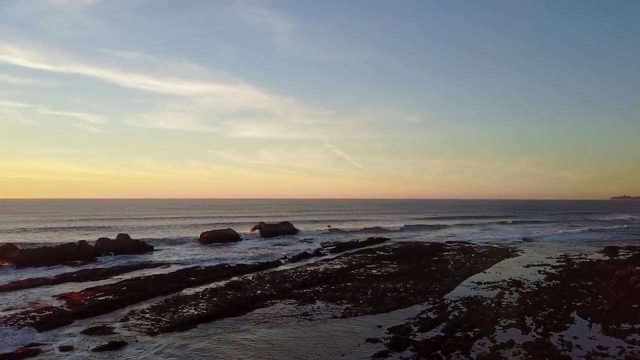 97% of this water is composed of our oceans and seas. Let's take a look at the ocean. Your face is delicate, so I just feel fine. Your face is delicate, so I just feel fine. Your face is delicate, so I just feel fine. 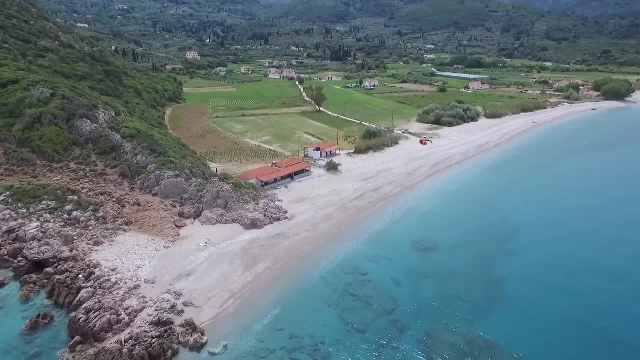 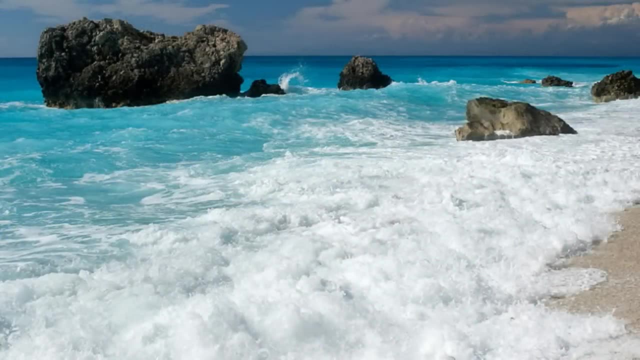 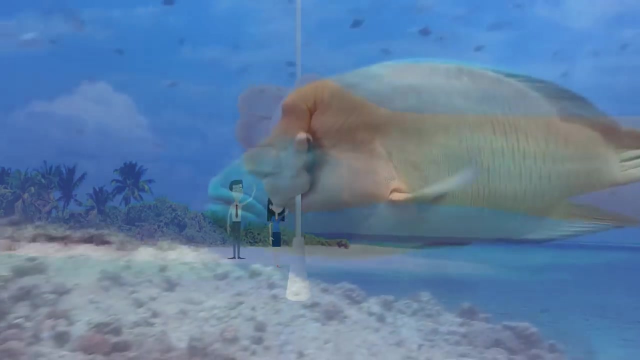 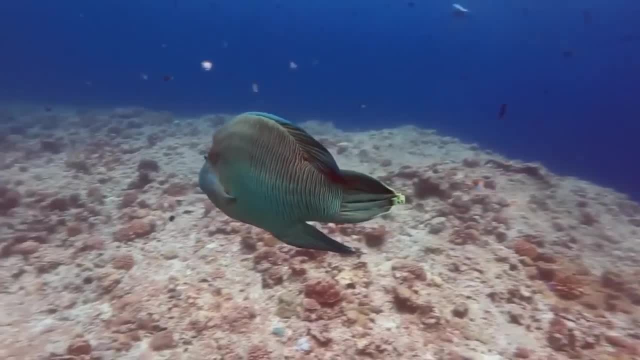 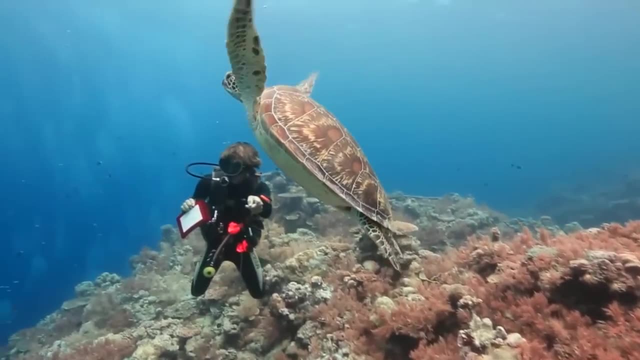 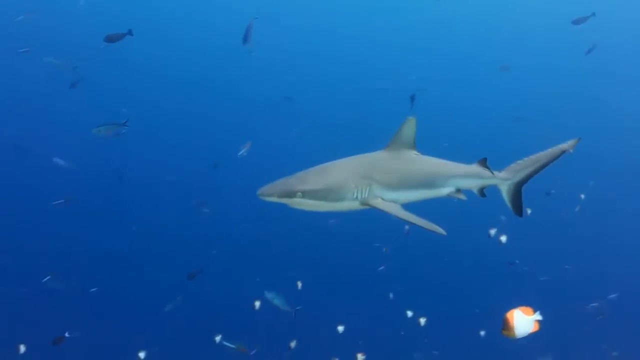 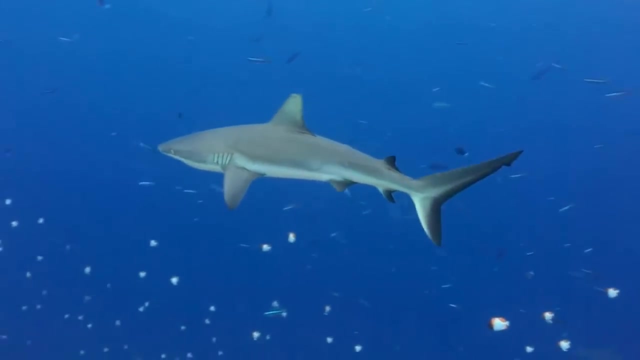 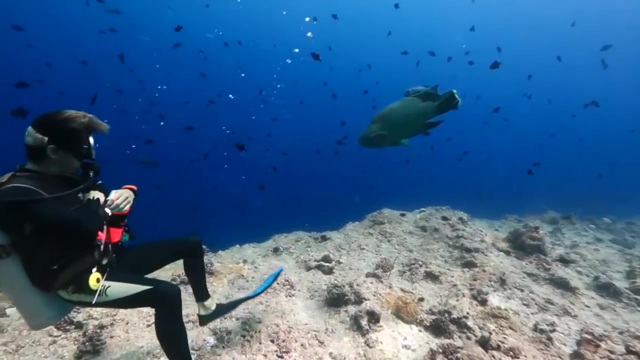 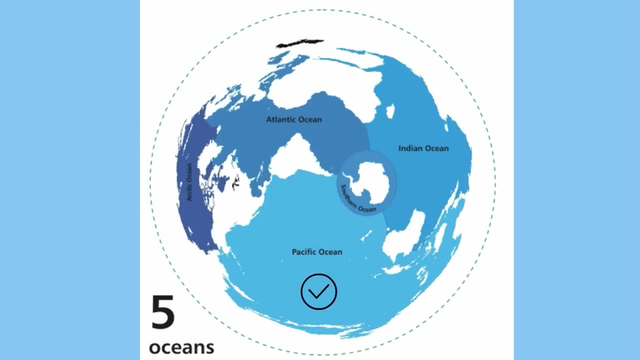 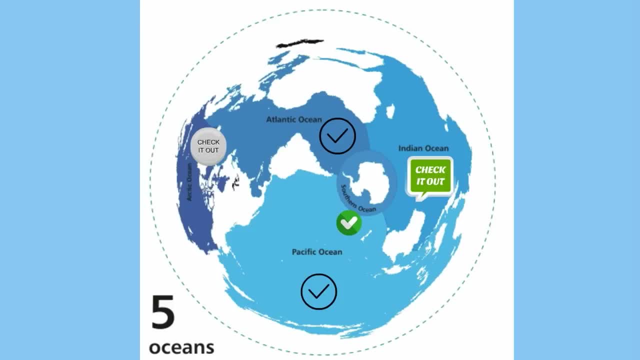 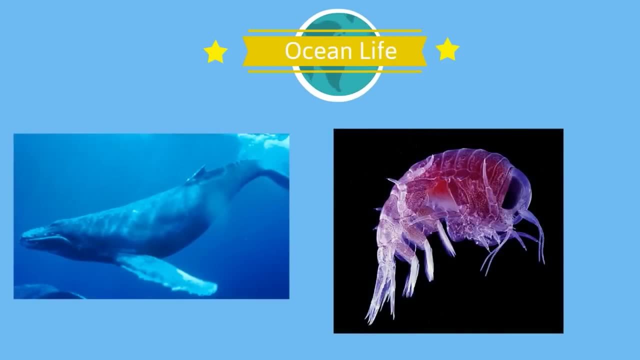 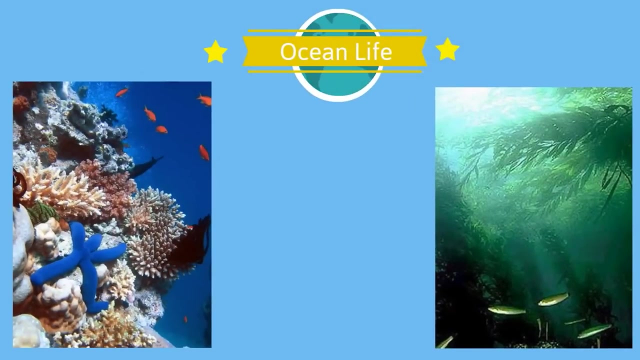 seas. The ocean is teeming with life. It includes animals as large as a 40-foot humpback whale and as small as microscopic plankton. It also includes a huge variety of plants and coral reefs that stretch for miles. It also includes the largest mountain range, called the Mid-Ocean Range. 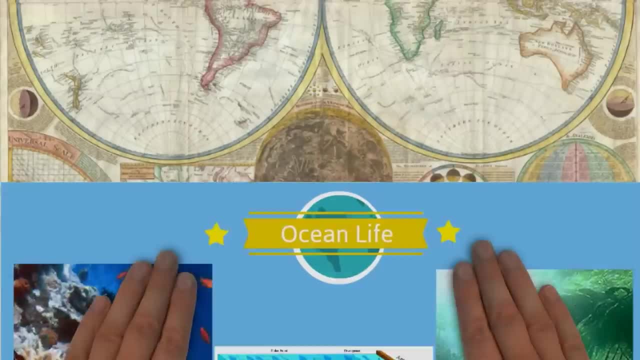 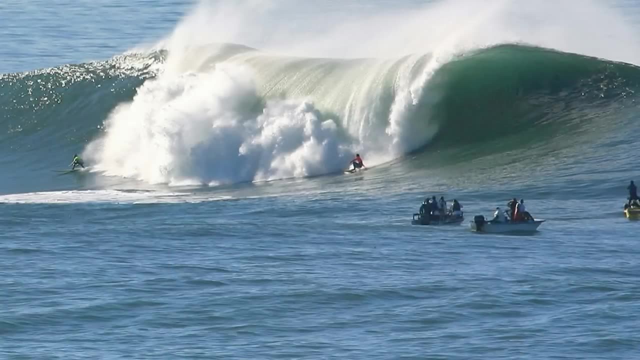 The ocean impacts our weather and has been used for years as trade routes. We play on the beaches of oceans and wonder what can be found in the deep trenches, like the Mariana Trench, which is 32,000 feet deep. Although we're fascinated with the ocean, we've only explored about 5% of the ocean. 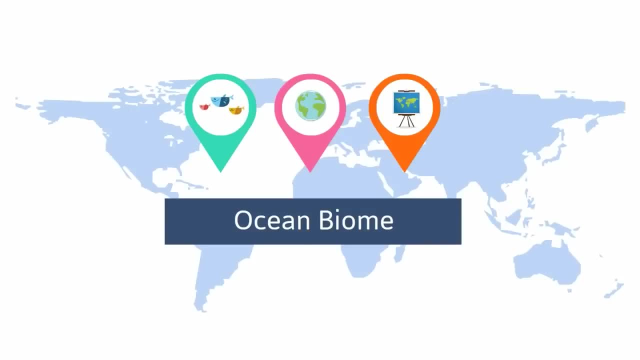 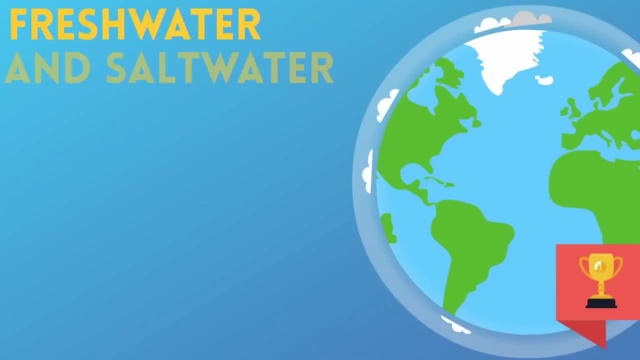 So there you have a quick overview of the ocean. Thanks for watching. We'll see you next time. Take care, Bye. The ocean is a large ecosystem of the ocean. It is a body of water that has fresh water entering and is also open to the ocean. 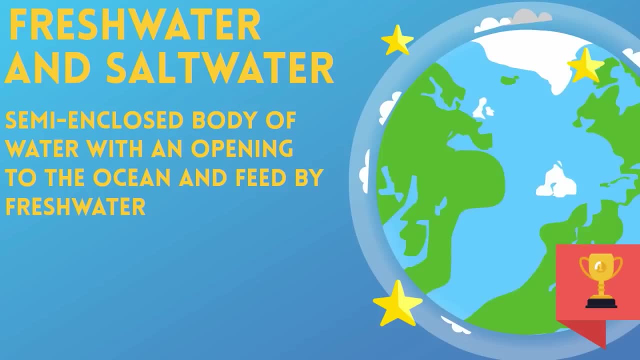 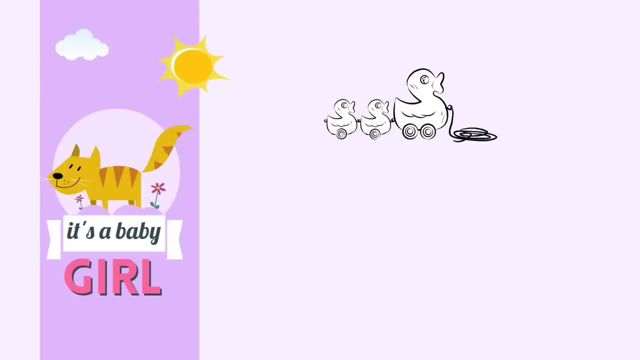 It is a semi-enclosed coastal body of water and it is connected to the open sea. Also, this salt water is diluted when fresh water from land drains into it. Estuaries have been called the nurseries of the sea because they provide a safe environment. 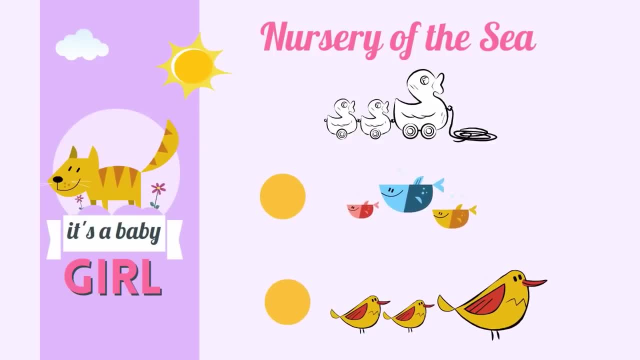 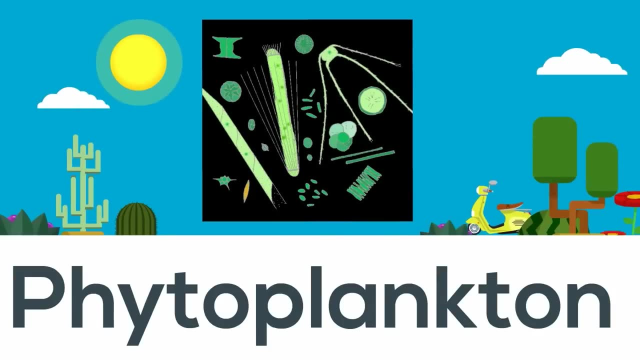 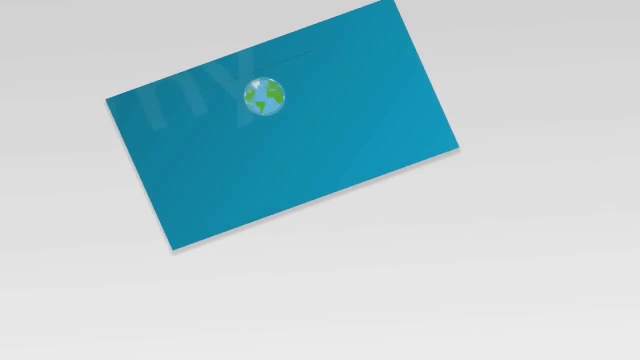 for fish and birds and other wildlife to raise their young. Estuaries also have producers called phytoplankton which help the food chain and provide food for many of the wildlife. Estuaries also help because they filter sediment and pollutants from the water before it flows. 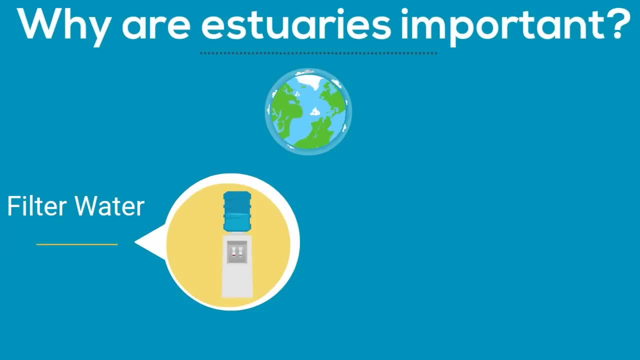 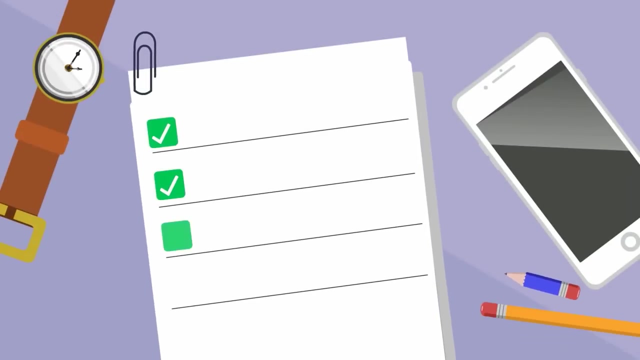 into the ocean. Estuaries are also important because they buffer the ocean and the land, and they can help decrease the effects of flooding and storm surges. Estuaries can be classified according to their geological features. The classifications include coastal plain estuaries. 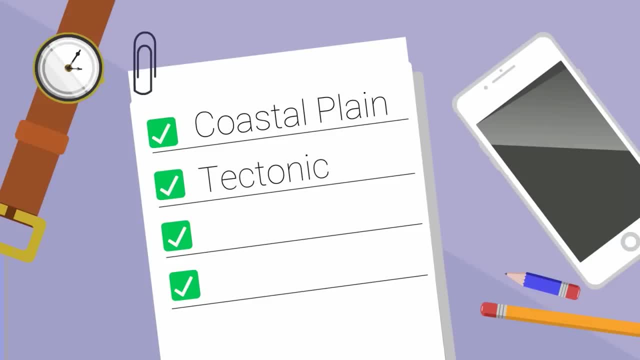 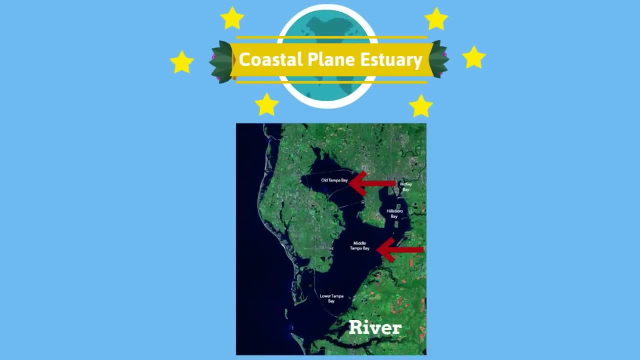 • Tectonic estuaries. • Bar-built estuaries and fjords. Coastal plain estuaries look like valleys with gentle sloping bottoms. Their depth increases toward the river's mouth. This type of estuary is common throughout the world. An example is Tampa Bay in the US. 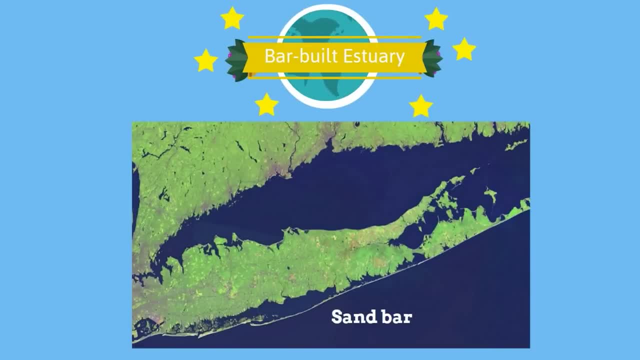 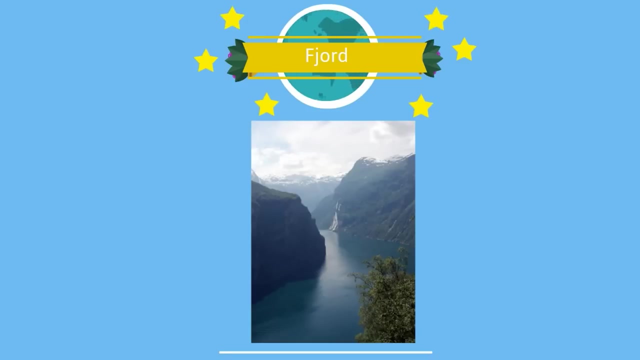 Fjord estuaries are formed when sandbars build up along the coastline and they partially cut off the waters behind them from the sea. Fjord estuaries are narrow, with steep sides, and are usually straight and long. Fjords are found in areas that have been covered by glaciers. 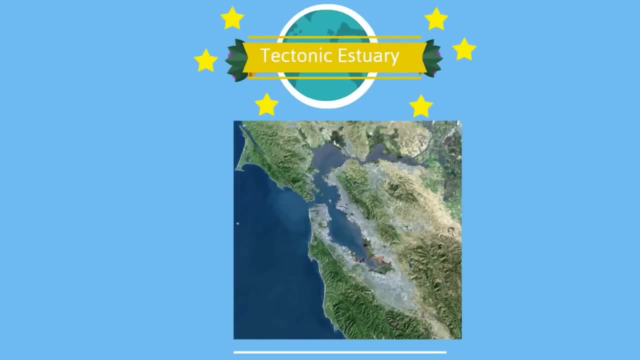 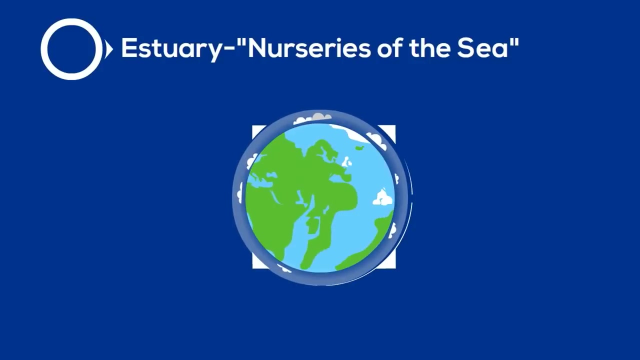 And finally, tectonic estuaries are created when the sea fills in a hole or basin that's formed from sinking land. San Francisco Bay is a good example. So there we go: estuaries, the nurseries of the world, places where fresh and salt water. 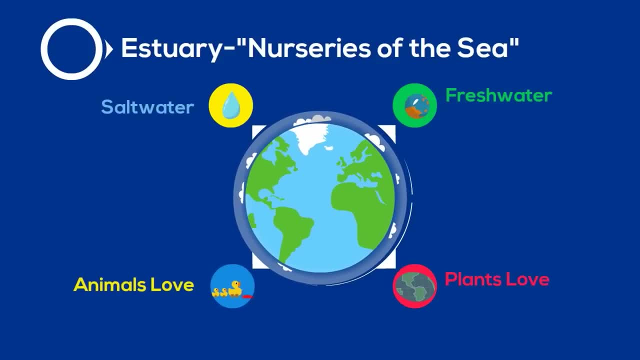 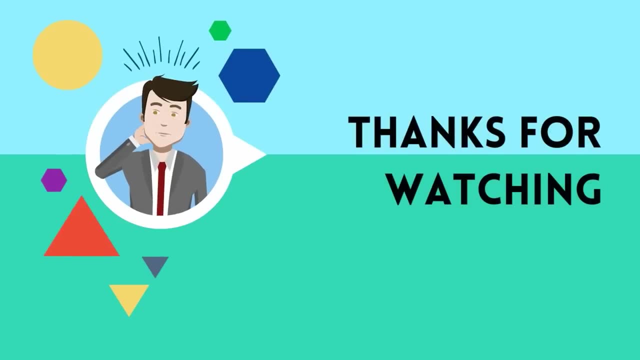 mix together what plant and animals love. Thanks for watching, and MooMooMath uploads a new math and science video every day. Please subscribe and share. 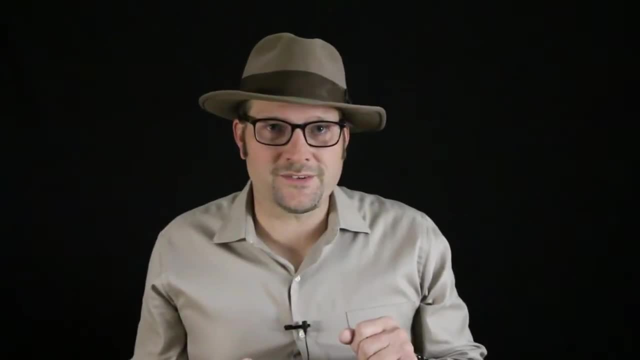 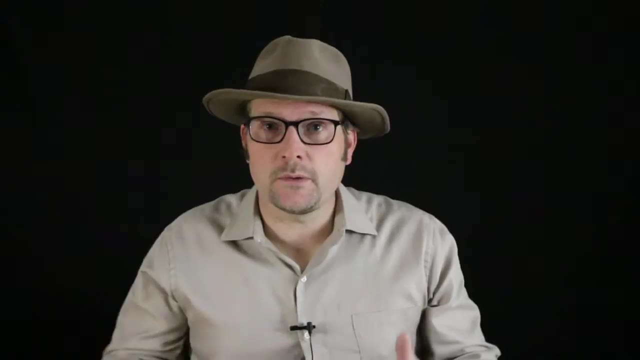 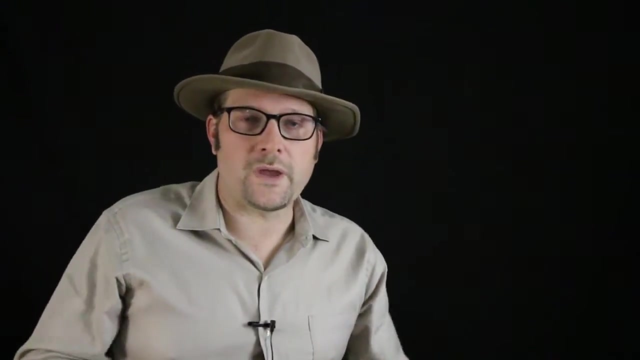 Welcome to Utah State University's Vertebrate Paleontology course. My name is Benjamin Burger, and in this video we will evaluate the evidence for the relationships between different groups of lizards and their origins. Most of today's lizards belong to a single monophyletic group. 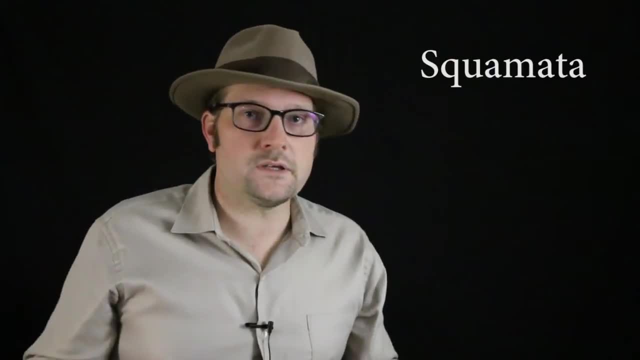 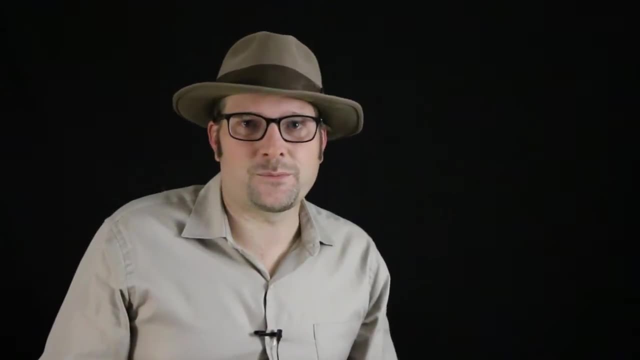 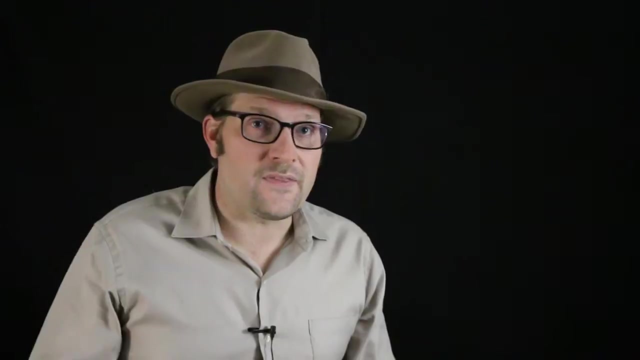 called the Squamata, which arose during the early Jurassic from an earlier diapsid reptile. Well… almost all of today's lizards belong to this group. There are two living species which lack the characteristics of the Squamata, and these two living species.